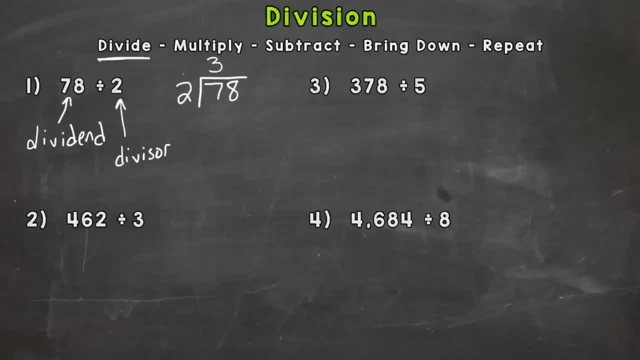 do that, So we divide it And that 3 needs to go right above the 7.. Keep things lined up Now. we need to multiply. We take this 3 and we come back around And we do 3 times 2, which is 6.. Then we 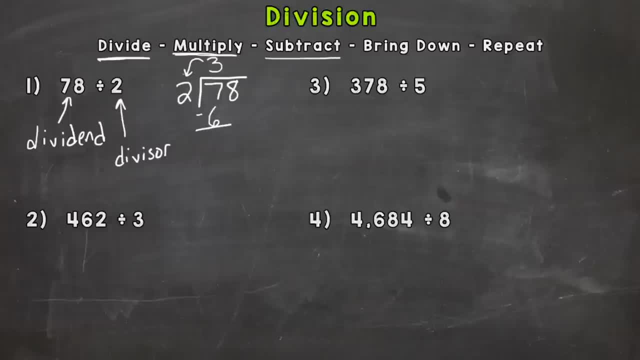 subtract 7 minus 6 is 1, and then bring down. So the next step is to divide. So we have to divide 3. the number we bring down is the next number. so next to the seven we have an eight. that's what we bring down, and I like to use an arrow. that way I it helps. 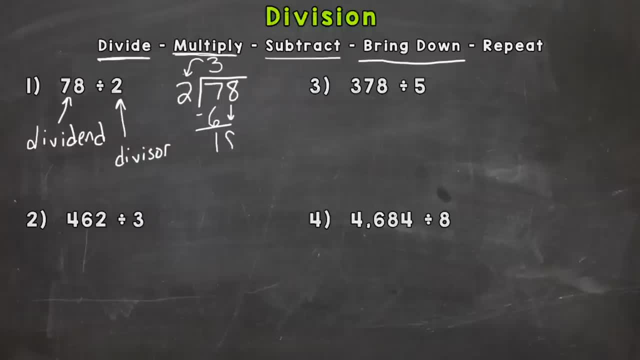 me keep things lined up and organized. so I bring down this eight and now I need to do a repeat of the steps, so I come back over here to divide, so I start everything over. so I need to do 18 divided by 2 now. so how many whole groups? 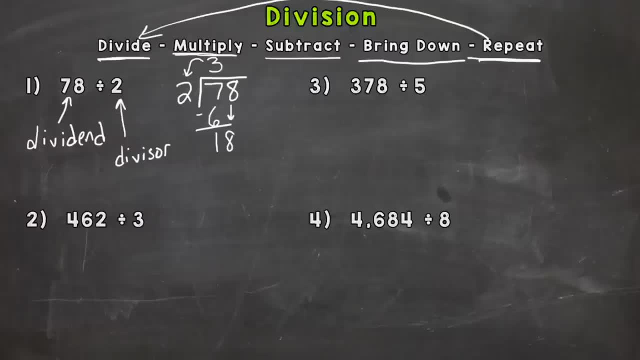 of 2. can I pull out of 18? and the answer to that is 9. then I multiply 9 times 2 is 18. subtract 18 minus 18 is 0 and then bring down. but I went all the way over to my ones place and I do not have anything else to bring down, so this: 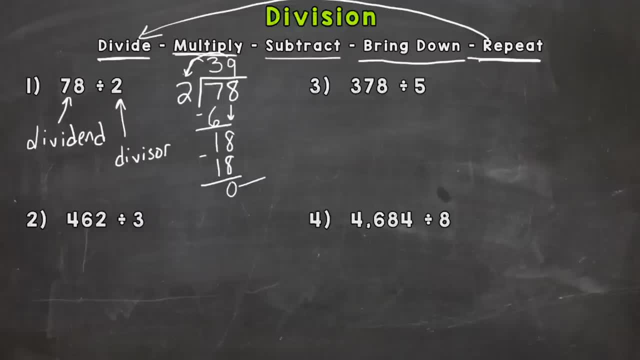 means I am done with the problem, and this 0 tells me I do not have anything left over. so that means no remainder. the quotient or answer is 39, and that word quotient, that means an answer to it, to a division problem. so let's take a look at number. 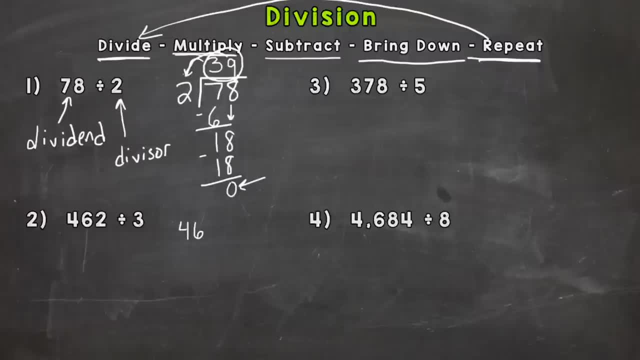 2. here we have 462. that's our dividend divided by the divisor, which is 3. so the first step is divide. we need to do 4 divided by 2, which is 4, divided by 2, which is 3. so the first step is divide. we need to do 4 divided. 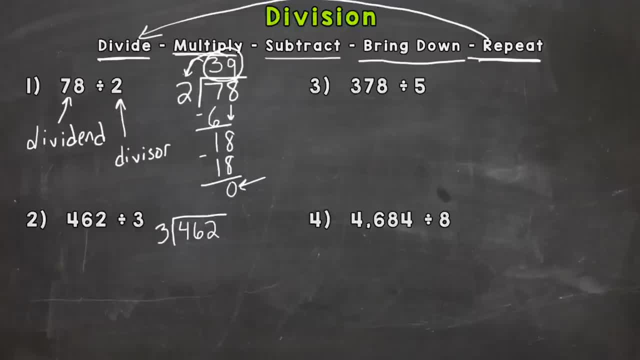 by 3. how many groups of 3 can we pull out of 4: 1? then we multiply 1 times. 3 is 3. subtract 4 minus 3 is 1. then we bring down the next number, which is the 6 and. 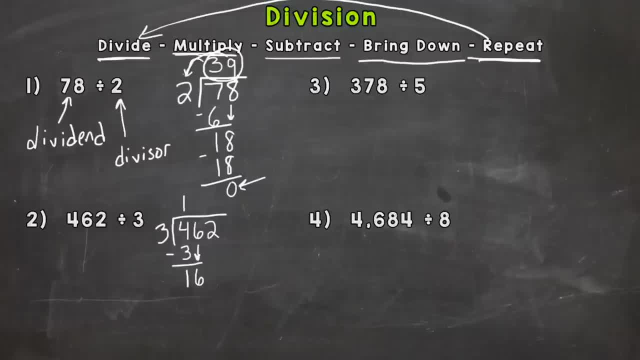 we start everything over. so we divide 16 divided by 3, how many groups of 3 can we pull out of 16 or make out of 16? and that's 5, 5 times 3. we multiply now, 5 times 3 is 15. subtract 16 minus 15 is 1, and then bring down the 2, so start over. 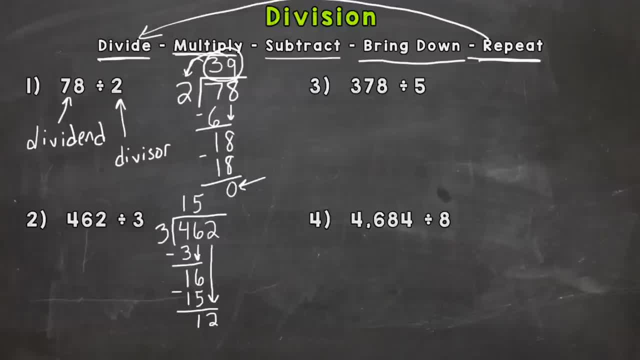 we have 12 divided by 3. how many groups of 3 are there in 12? how many groups of 3 can we make out of 12? and that answer to that is 4. so now we come back around: 4 times 3 is 12. 12 minus 12 is 0. we went all the way over to the ones place, so we 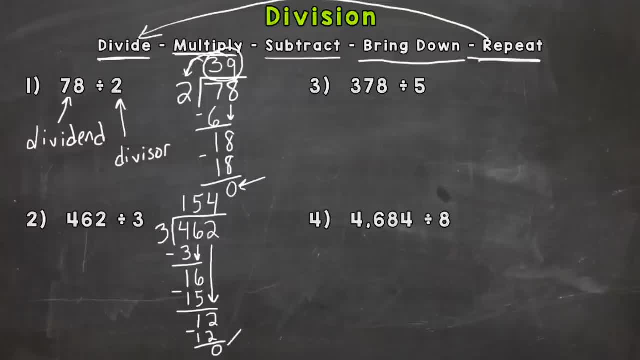 don't have anything else to bring down and this 0 tells us we have a remainder of 0, nothing left over. it divided perfectly into to give us a whole number, so the quotient or answer is 154. one of the main keys or biggest components of getting a correct answer is having 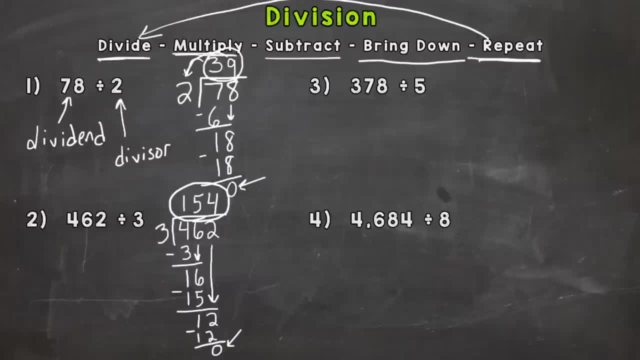 everything lined up and staying organized. so one thing I would suggest: if you're having trouble staying lined up and if your problems start to curve or you're not sure what to bring down next or things aren't lining up, take a look at the answer and you'll see that everything is lined up and you can see. 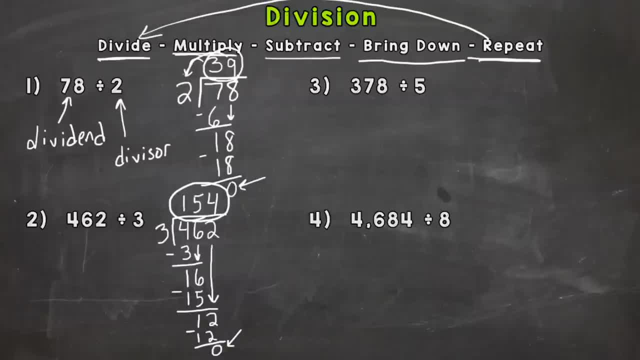 a piece of lined paper and turn it sideways and use the blue lines as your guides and to help keep you keep everything lined up as you go through the problems. so let's take a look at number three, and this one's a little different. so we have 378 divided by 5. so this one's a little different because we 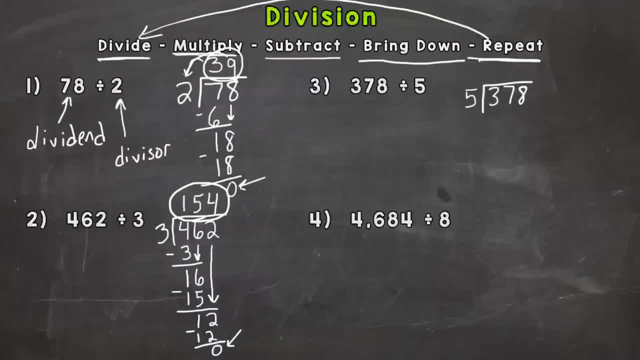 start with 3 divided by 5, which we can't do and get a whole number. so we need to do 37 divided by 5. so if you cannot do 3 divided by 5 or whatever that first number is, you need to hop over to the second, and now we have a two digit. 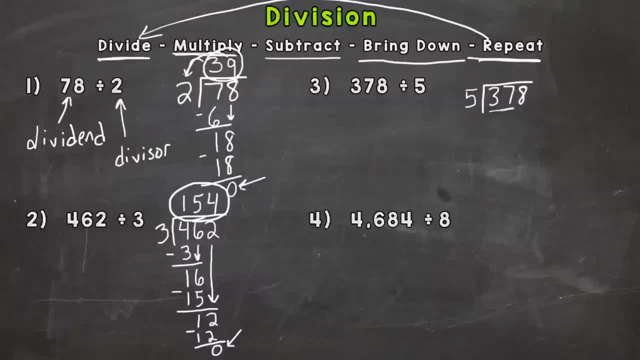 number 37. so we need to do 37 divided by 5. how many groups of 5 are in 37? well, 7, and it's very important where you put this number: that 7 needs to go above the 37, not the 3. 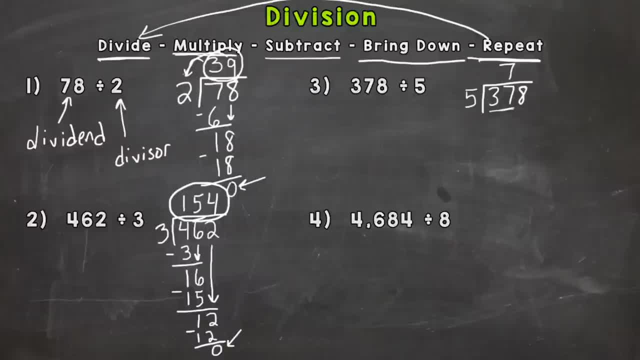 you have to have it lined up with the 37. so now we multiply, we come back around. 7 times 5 is 35. subtract we get 2, and now we bring down the 8, so now we have 28 divided by 5. how many groups of 5 can we pull out of 28? well, 5, 5 times 5 is 25. 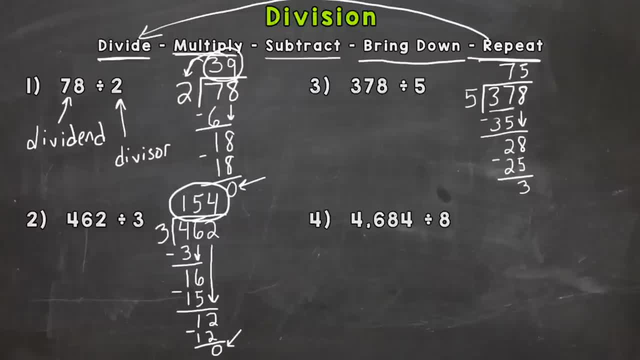 subtract and we get a 3. we went all the way over to the ones place, nothing else to bring down, so this 3 is a remainder, it's a number left over. okay, so when we did 378 divided by 5, it doesn't work out into a perfect whole number. we have three. 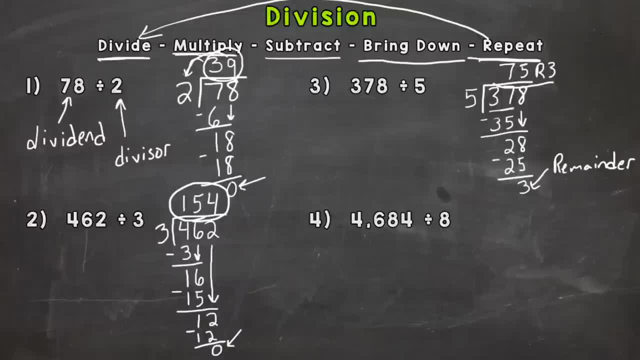 left over. so the answer is 75 remainder 3. so let's go to number 4. here we have a 4 digit dividend and a single or one digit divisor, so 4684 divided by 8. so let's start with: how many 8s can we pull out of 4 or 4 divided by 8? we can't do. 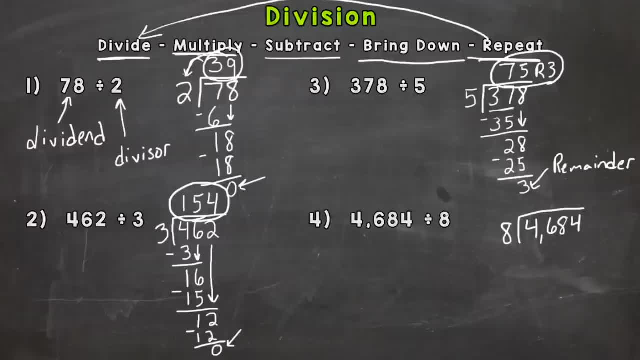 that and get a whole number. so we need to jump over to the 46. so 46 divided by 8 is 5 and that gets us to 40. so we multiply now 5 times 8 is 40, subtract 46 minus 40. 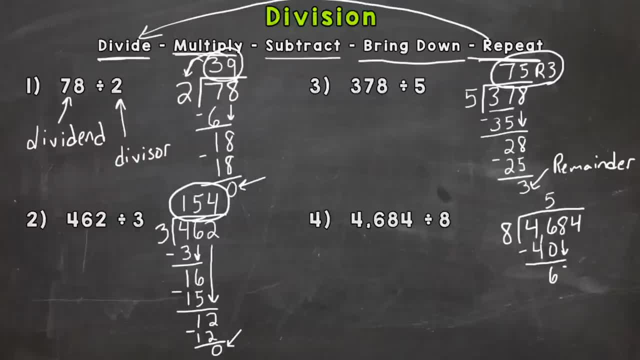 is 6, and then we bring down the 8, so we have 68 divided by 8 and 68 divided by 8. we can do 8 8 times 8. 64 subtract 685000 divided by 8, we have our자는 and.